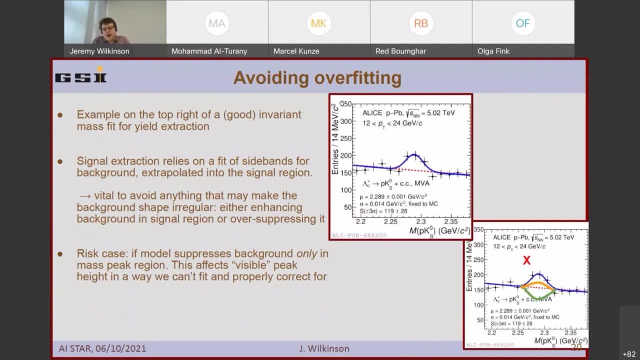 And what we want to do in particle and nuclear physics experiments is to probe exotic states of matter where these quarks are, And what we want to do in particle and nuclear physics experiments is to probe exotic states of matter where these quarks are. So one particular thing that we need to be careful of when we're making precision measurements in particle physics is that we don't want to make an overfit of the data. 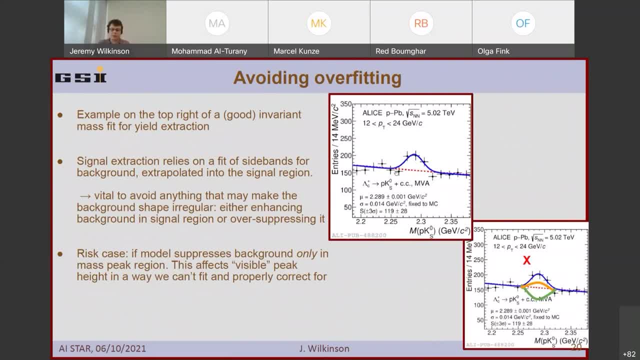 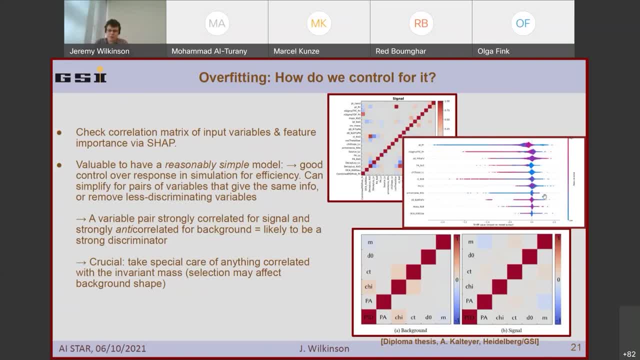 And then we will have a peak- typically a Gaussian- of our real signal. sitting on top of this, We can also remove variables that are less well discriminating, And then the crucial thing is that we have to take special care of anything that has a correlation with the invariant mass of the overall particle, to avoid the effect that I mentioned in the previous slide. 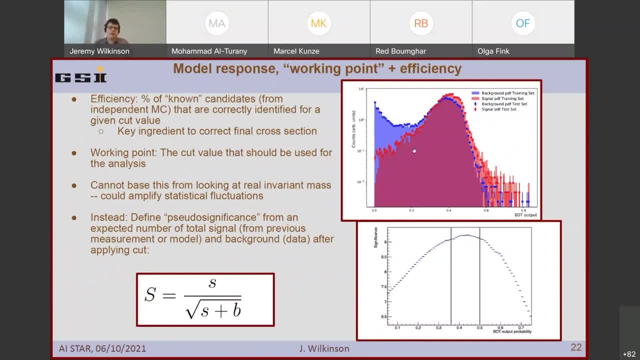 So, then, what we determine is the efficiency, is the percentage of known candidates from an independent Monte Carlo that are correctly identified for a given cut value. This on the top right is an overview of a typical BDT response that we have for a simple signal background training, where the background is shown in blue and the signal is shown in red. 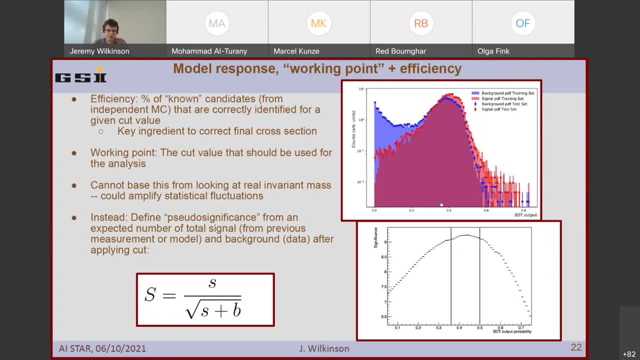 And we'll take the proportion of this above the cut value that we apply on the data to figure out what our efficiency is and then correct for this in order to get out the actual proportion that was produced in the first place, Then to determine where we want to set the cut for this. we don't want to base this from looking at the real invariant mass distributions for every individual cut value, since this could amplify statistical fluctuations. 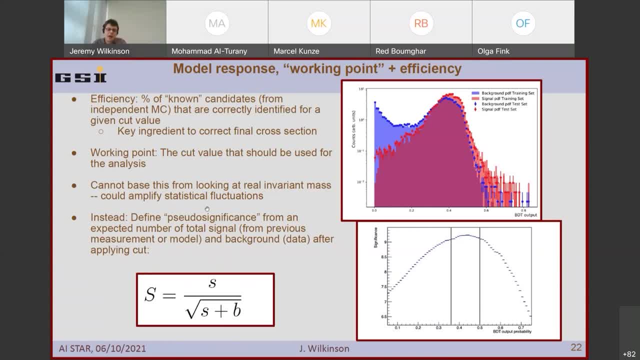 So instead we define this pseudosignificance variable from an expected number of total signal from either a previous measurement or from models, and then the background from real data after applying the cut. So this then gives us. This then gives us an estimate of where our likely best region would be to apply the cut in order to get the best statistical significance. 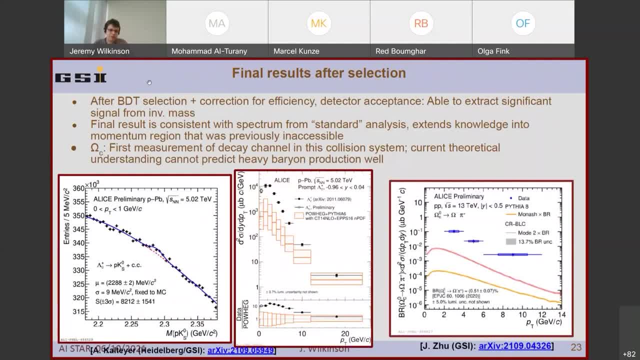 And then this brings me to the final results after the selection. So, after making this BDT selection and correcting for efficiency and detector acceptance, we're able to extract a quite significant signal from the invariant mass distribution at the lowest PT region, where we particularly 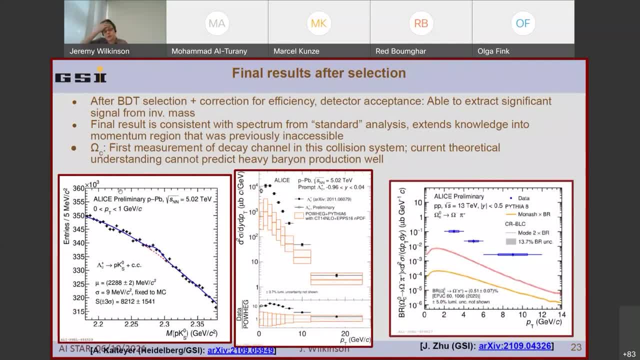 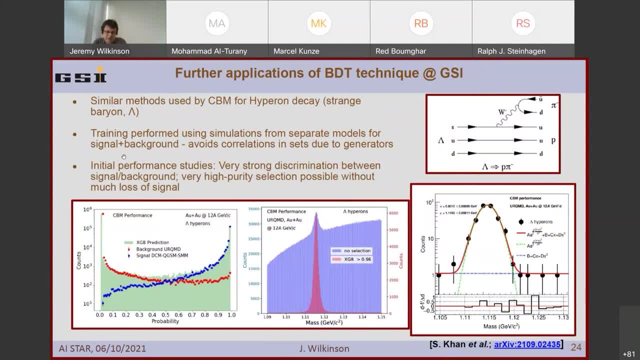 In this case there isn't any real data yet because the detector is still under construction, but we can perform training still using background that's generated by a model that's independent from the signal generation, And the initial performance studies of this are showing that there's a very strong discrimination between the signal and background, either before the selection in blue and after selection in red. 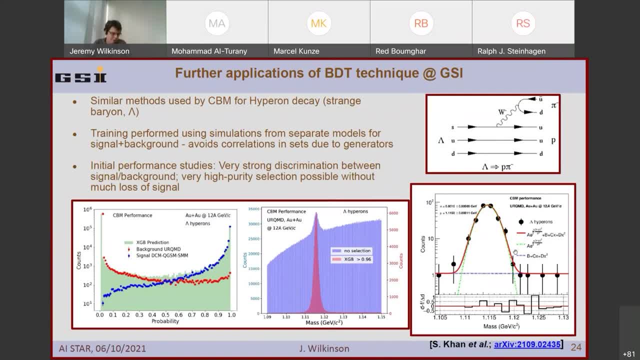 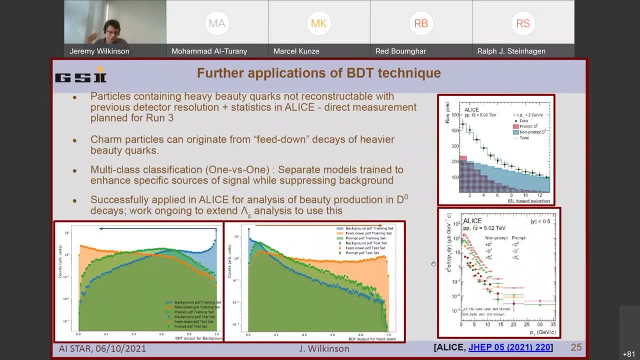 And then this allows, Allows us to make a very high purity selection without much loss of signal, And then we can push the techniques also towards multivariate techniques in order to distinguish the initial sources of the particles that we measure. So we perform a one-versus-one training of separate models for background. 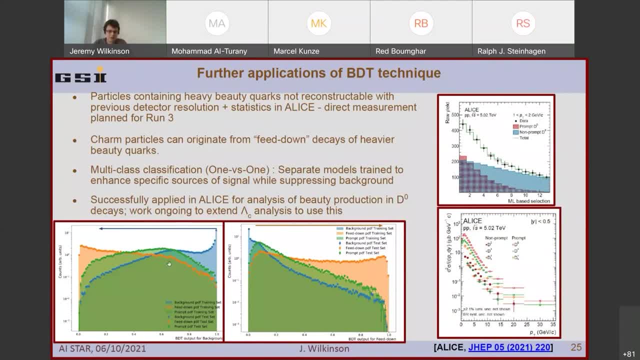 prompt, which is from a charm quark, and feed down, which is from a beauty quark, And we can make a simultaneous cut on these models in order to both suppress the level of background while enhancing the level of feed down production, And this has been successfully applied for demisons elsewhere in the ALICE collaboration and work is ongoing at GSIE to extend the lambda C analysis to use this. 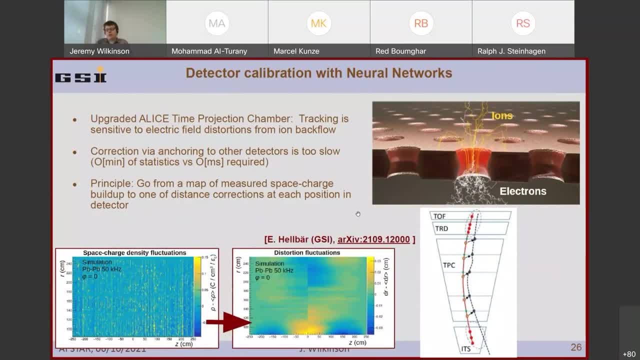 And then I want to briefly touch on, so not just on the data analysis, but also how we use machine learning techniques in order to calibrate our detectors. So we've recently made upgrades to the ALICE time projection chamber. for the upcoming run, three of the LHC. 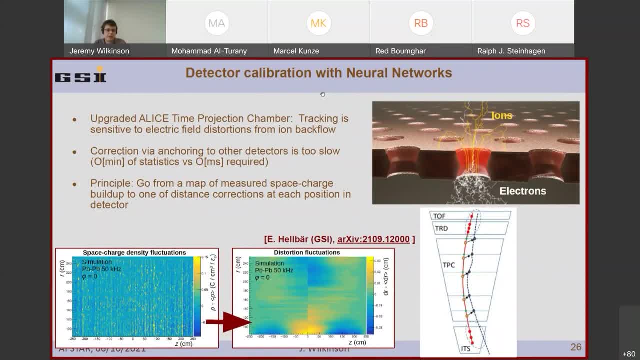 So the tracking in this new detector is quite sensitive to distortions in the electric field from ion backflow, which can then lead to a distortion of the track that we end up reconstructing in the detector, And the one method that can be used to correct for this is to anchor tracks to the response from other detectors. 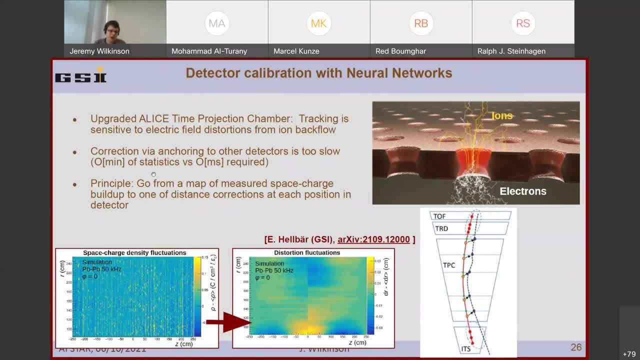 But typically this requires statistics on the order of minutes to be able to make this correction, while the fluctuations that we're dealing with are on the order of milliseconds. So what we want to be able to do is take a map of measured space charge, build up 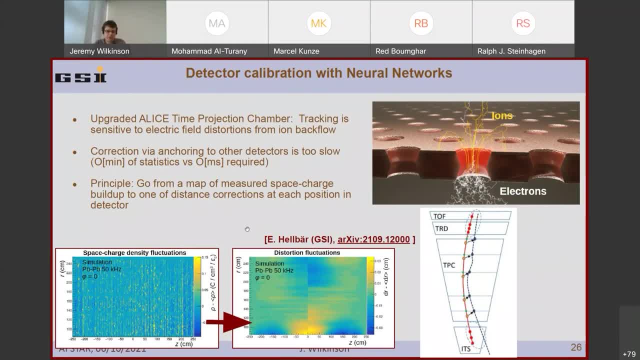 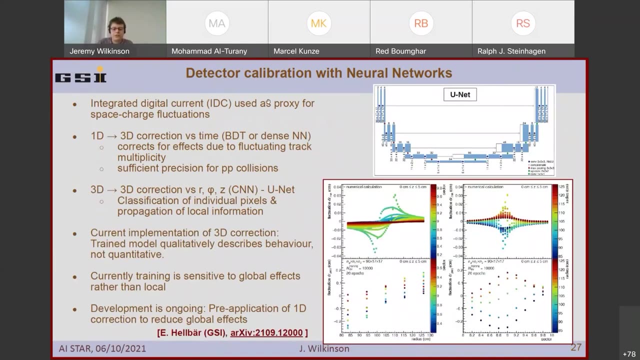 in the detector and instead map this to distance corrections that we can apply at each position in the detector to get reliable tracking information out. So what we use for this is the integrated digital current, or IDCs, in various regions of the detector. 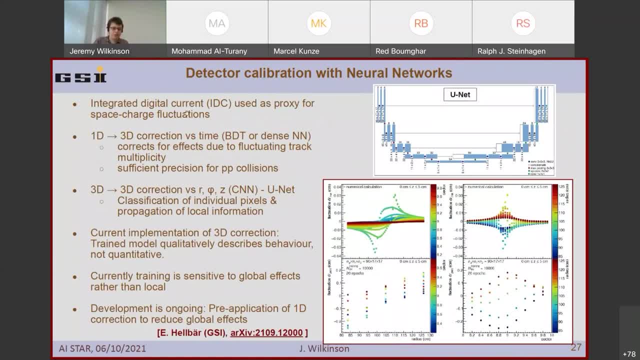 And this can be used as a proxy for the fluctuations of this so-called space charge build up. So we can either perform a one-dimensional correction versus time using BDTs or dense neural networks which allow us to correct for effects due to the fluctuating track multiplicity. 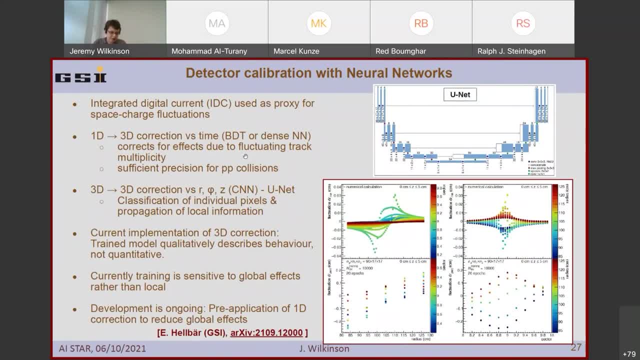 And this gives sufficient precision for proton-proton collisions. For higher multiplicity collisions, such as lead-lead, we need to be able to perform a 3D correction versus the radial position and also the angle and Z position, And then this would be performed using a convolutional neural network known as a U-net. 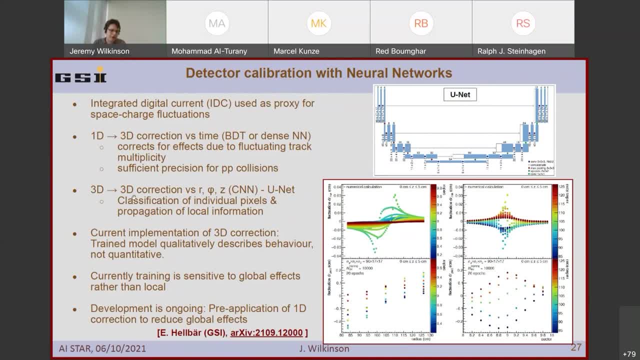 which allows us to classify individual pixels and propagate really the local information from each detector region. The current implementation of the 3D correction is shown on the bottom right. So on the top we have a numerical calculation of the fluctuations versus the machine learning response on the on the bottom plots. 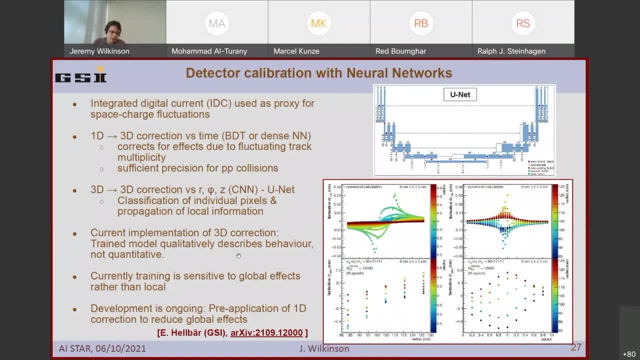 So what we're finding at the moment is that the trained model is qualitatively describing the behavior, but is not really quantitatively able to describe it so far, And what we see from this is that, really, the training at the moment is sensitive to more to global effects rather than local effects. 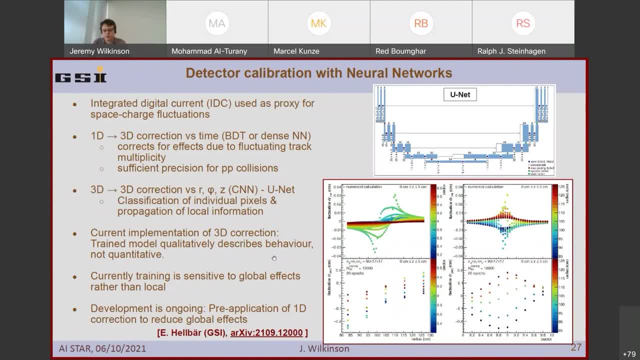 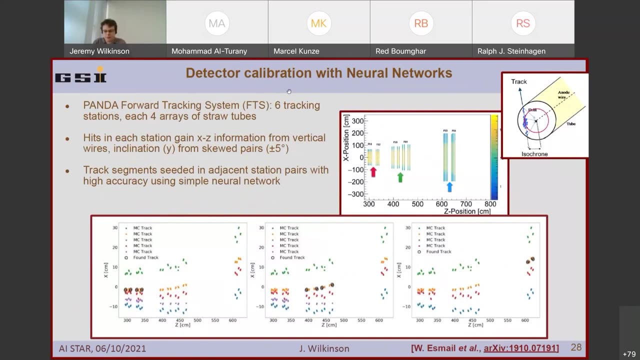 But development is still ongoing on this. So, for instance, the pre-application of the one-dimensional model, one data correction to reduce the global effects prior to the, the 3D training, And then, finally, we can also consider the reconstruction of tracks in the future Panda experiment. 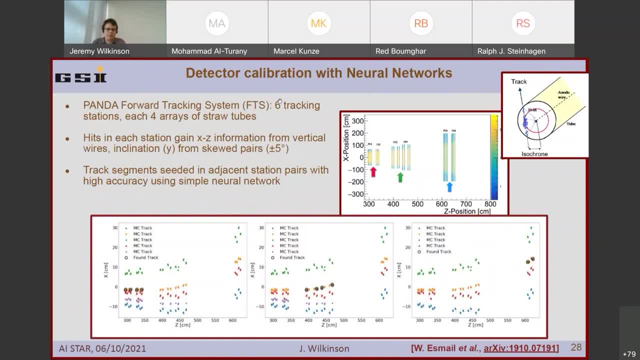 So the forward tracking system of Panda is formed of six separate tracking stations at different positions in Z, which are arrays of these straw tubes. The straw tube itself can only measure a signal in the center of it, but then we can use combinations of these straws to determine better the the actual spatial position. 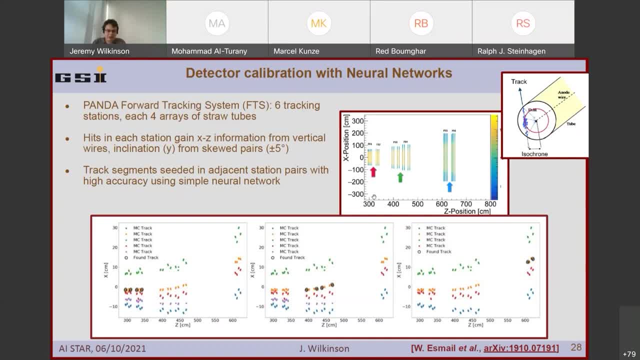 So you have hits in each station that have XZ information from the vertical wires and then the inclination of the track from pairs of skewed wires in the middle. The track segments are seeded in adjacent pairs of stations using a simple neural network and you have an. 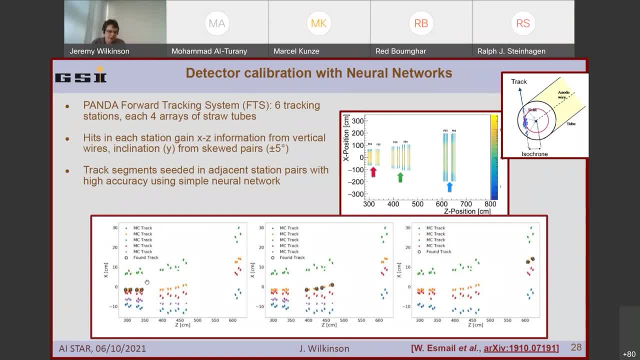 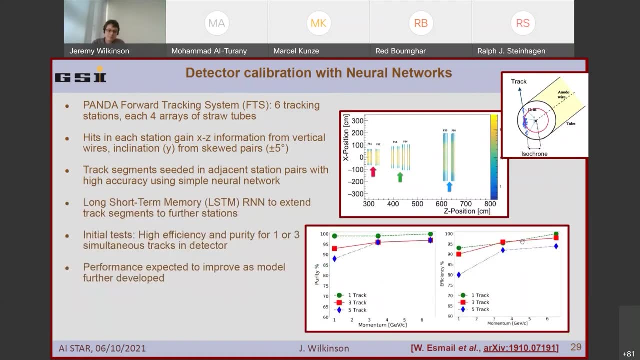 illustration of the, the performance of this so far. So the the orange track is reconstructed with the, the black circles in each of the individual pairs of tracking stations with quite high accuracy using a simple neural network, And then we can use also a long short-term memory. 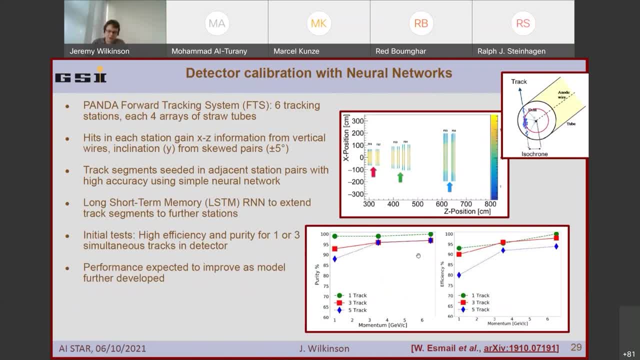 recurrent neural network to extend these track segments to the further station. So this was covered a little bit in the in the previous talk, And initial tests of this are showing quite high efficiency and purity of the reconstruction for one or three simultaneous tracks in the detector, and then the performance for larger numbers of tracks is expected to improve as the model is further developed. 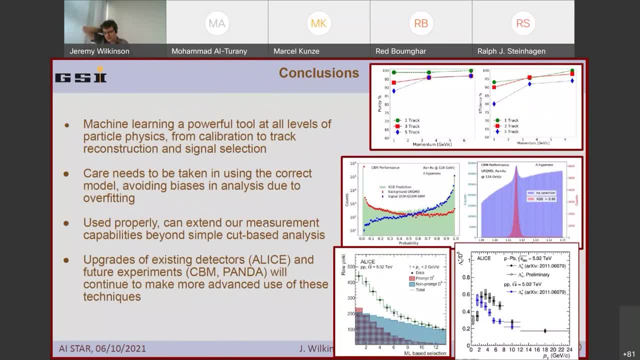 So this brings me to my summary. So with it's a hot and increasingly growing topic in particle and nuclear physics to use machine learning at all levels of our reconstructions, So from the initial calibration of our detectors to the track reconstruction and then our final signal selection. 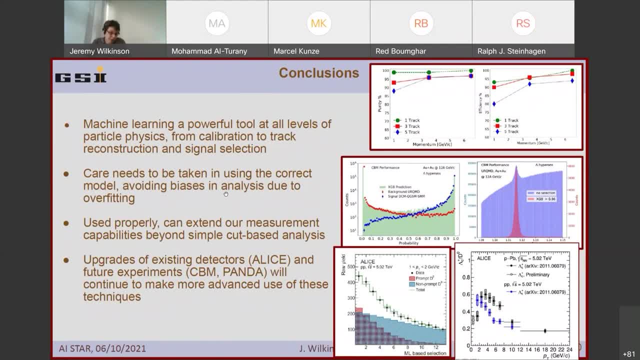 We obviously need to take care to use the appropriate models in order to avoid biases in our analysis due to potential overfitting. But, used properly, we can extend our measurement capabilities beyond the simple cut-based analysis that we were performing before, And then we have upgrades of the existing. 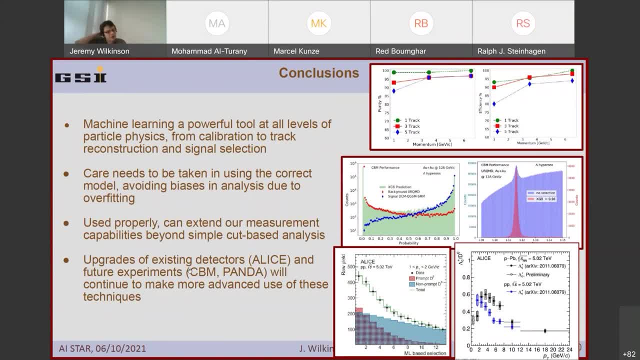 detectors and future experiments that will continue to advance our use of these techniques. So yeah, thank you for your attention. Thank you very much, Jeremy. We go to the questions Not too much, So one question from Ralph: How to estimate the statistical and systematic error of? 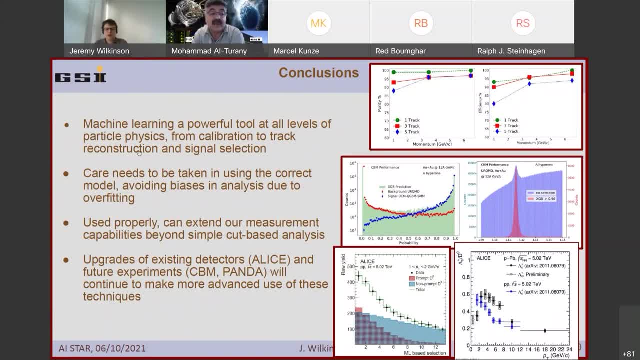 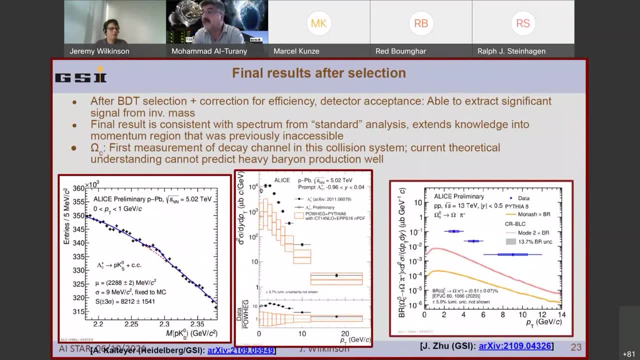 artificial intelligence based classification Bias with respect to reaching a classical five sigma, for example. confidence Right, yeah, So typically the the five sigma. The five sigma criterion is something that we apply if we are discovering a new species of particles for the first time. 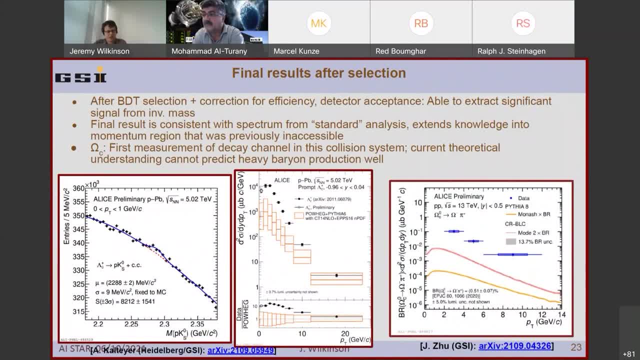 We can afford a slightly smaller number of sigma, So down to three sigma for an established particle species. So the statistical uncertainties, we typically take those from this invariant mass fit, where it's simply the counting uncertainty of the fitted signal over the background, And then in terms of the 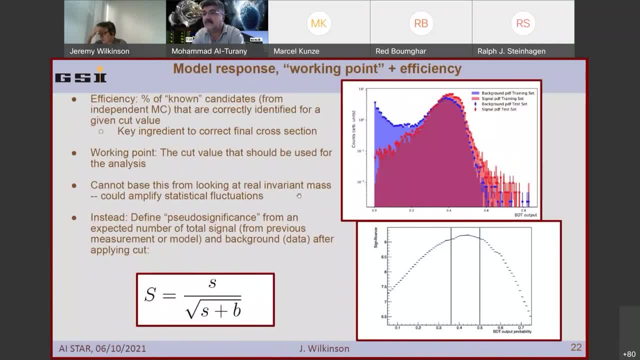 systematics from varying the cut. I didn't have time to really touch on this, but usually what we will do is around our chosen working point for the cut. we will vary the probability cut that we apply within some region and then see what the effect of this varied cut will be on the 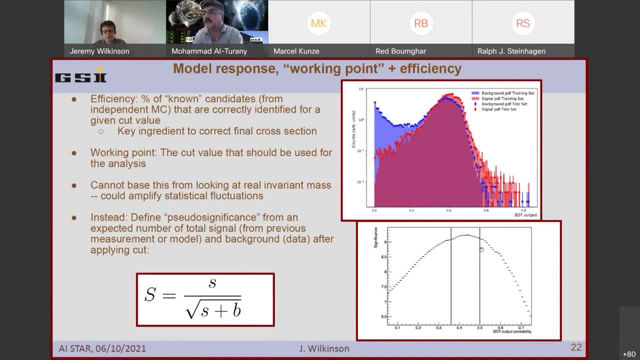 on the final reconstructed signal. So basically, it's a. it's a check to make sure that the the efficiency of our probability cut in the Monte Carlo properly reconstructs the effect that we see in real data, And it's quite similar to what we would do in. 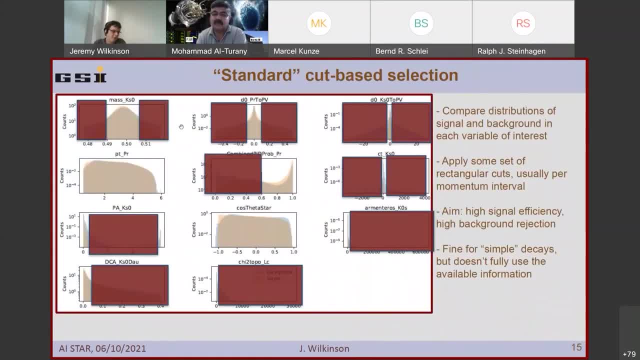 so even in the original cut based analyses we would perform a similar approach where we would be, instead of changing the probability cut and seeing how that affects the signal, we would be changing these individual cuts. So the approach there is relatively similar to a classical analysis, I would say. 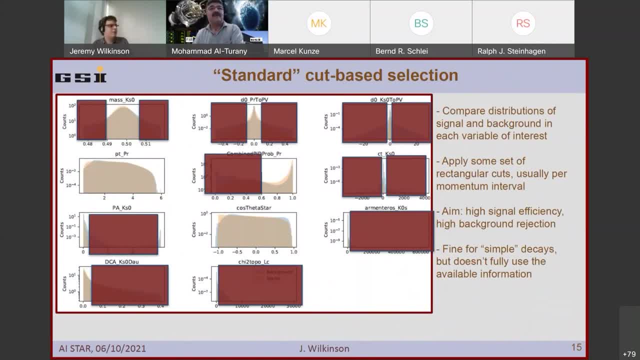 Okay, thank you very much, Jeremy, So as there are not too many other questions, so let's move to the next session of this meeting. Thanks, Jeremy.